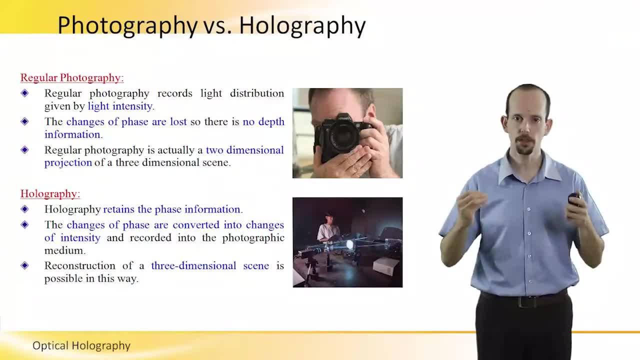 by light intensity and the phase information is lost. Because the phase information is lost, we cannot retain the depth information, And so regular photography is actually a two-dimensional project, And so regular photography is actually a two-dimensional project. And so regular photography is actually a two-dimensional project, And so regular photography is actually a two-dimensional. 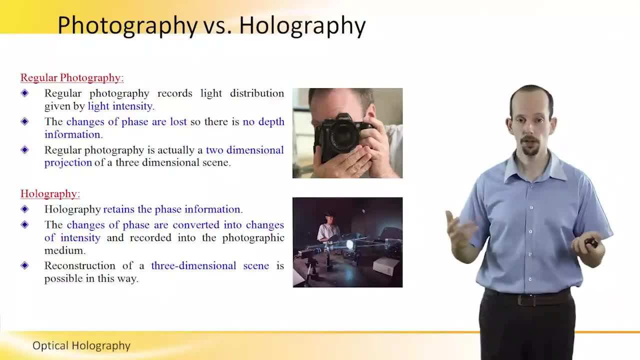 projection of a 3D scene. In holography we can retain the phase information because changes in phase are converted into changes in intensity using the holographic principle, which is based on the interference principle, And therefore the reconstruction of a 3D scene is possible. 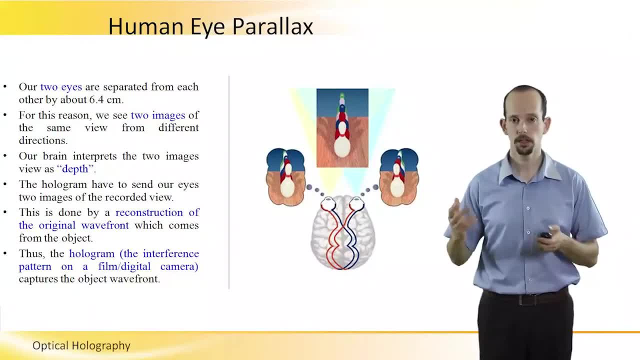 As you all know, we have two eyes And in an adult subject, the two eyes are separated from each other by approximately 6.4, 6.5 cm, And this is why we think we see 3D objects, Because our two eyes get different perspectives of 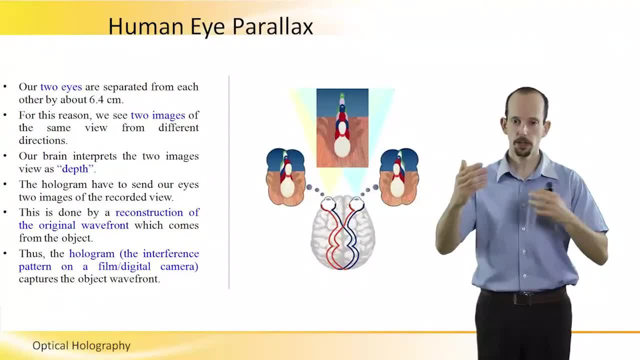 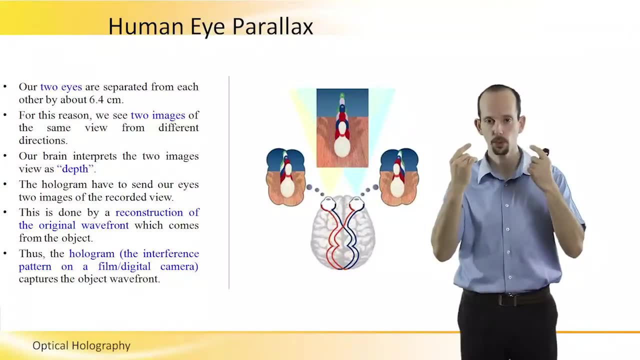 the 3D world. Our brain actually interprets these two images into depth, The hologram, have to send our two eyes to images, and this is not done, as done in stereoscopy, where we create actually two images and send them to each of our eyes and then we have probably have goggles with different. 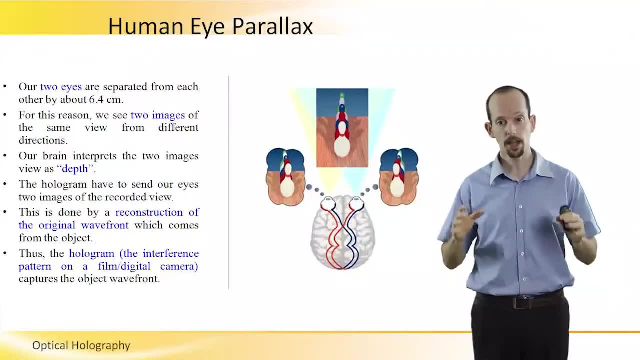 filters. this is done in a different way. this is done by a reconstruction of the original wavefront, the complex waveform which is recorded into the hologram using the interference. the film or the digital camera can actually capture the interference that is composed, that actually captures the amplitude and phase information, the original waveform that was emitted from the object. 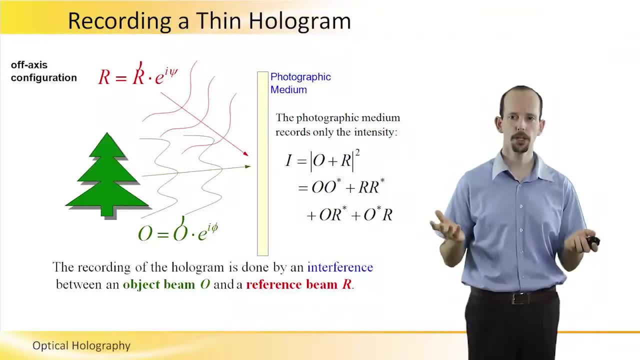 so this is how a thin hologram is recorded. we have a photographic medium, which is a regular film, which might be a little bit more dense than a simple photographic film, and then we have a 3D object object and we want to record the interference between the object beam O and the reference. 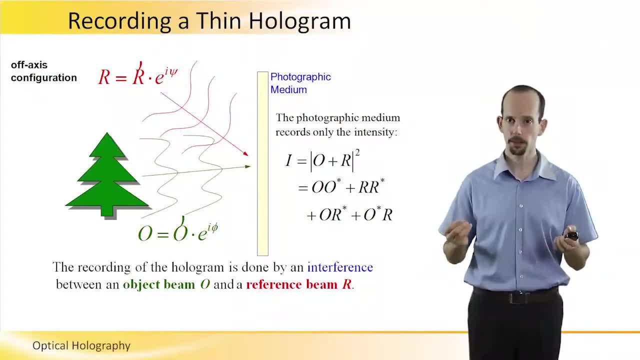 beam R, each of which is a complex wavefront containing an amplitude and a phase. So this 3D object emits a complex wavefront containing an amplitude and a phase, phi, And then, using interferometers for example, we interfere it with a reference beam that. 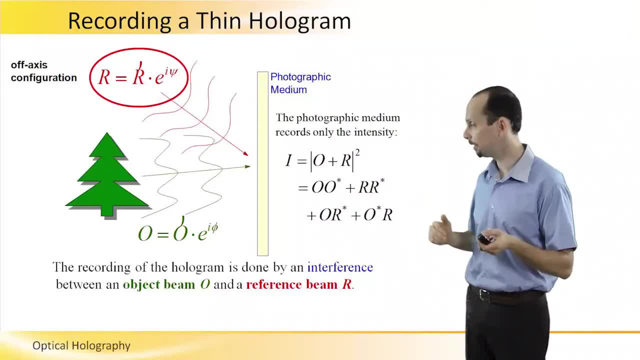 comes directly from the source, where these two beams are coherent to each other, which means that the optical path difference of the beams is smaller than the coherence length of the source, And this is called an off-axis configuration, because there is an angle between the reference. 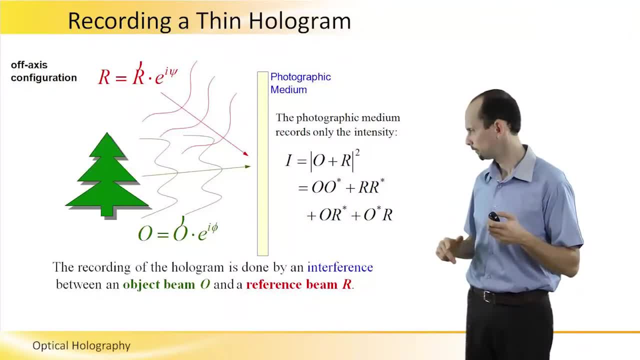 and the object wave. So the photographic medium records only the intensity. It might be a photographic medium and if we are talking about a digital holography, it might be a digital camera. So in this case it's a photographic medium, a photographic film and this photographic 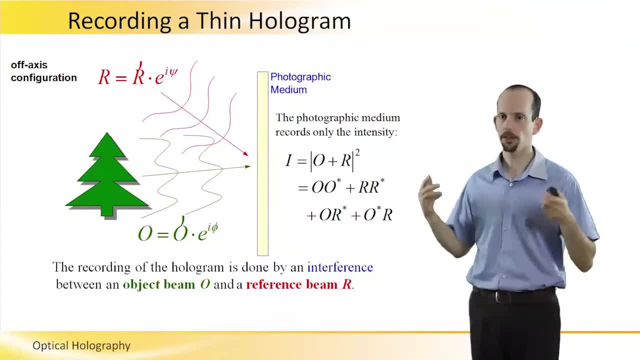 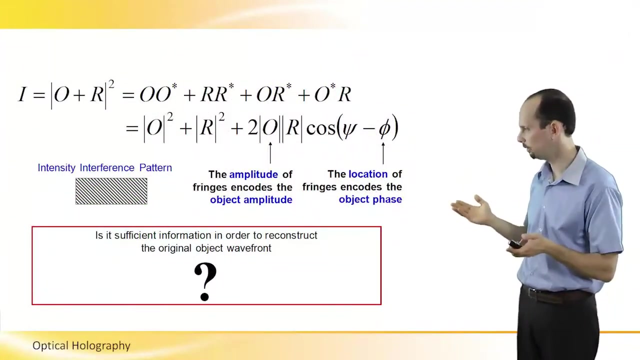 medium has. all kinds of detectors are sensitive to intensity only, and that means that as soon as as the superposition of these two waves hit the photographic medium, it makes absolute value square. So we have recorded the hologram which is a superposition between the object wave and 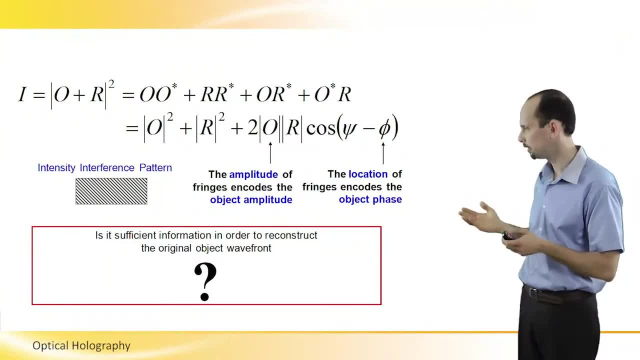 the reference wave and we get four elements. So the two first elements actually mean a DC- O- absolute value square- plus R- absolute value square. But the last two elements, because each of them- O and R- is a complex number actually. 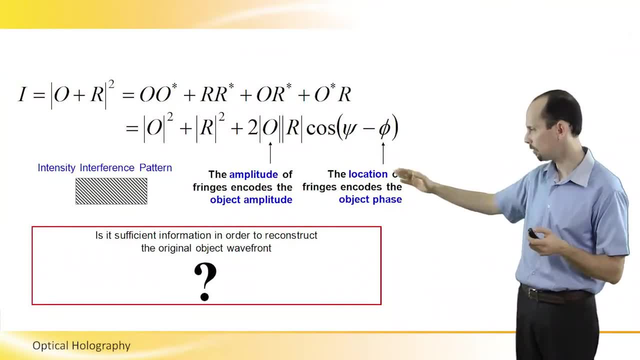 mean a cosine pattern And this cosine, if I'm looking on this cosine from the top, might look like that, because it's a cosine pattern And the amplitude of the fringes of the cosine, these fringes, encodes the object amplitude. 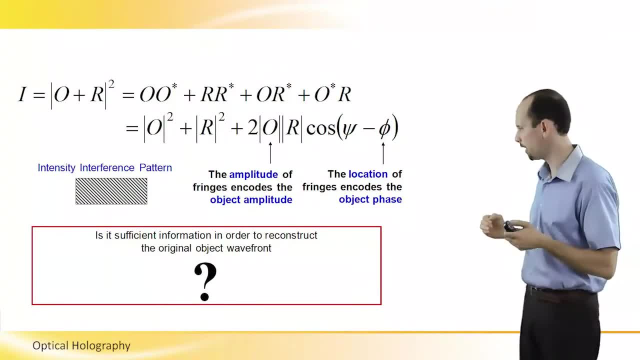 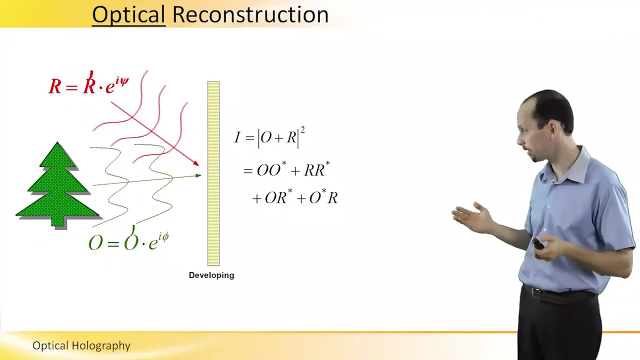 But the important thing is that the location of the fringes encodes the object phase. And the next question is: is this information enough in order to reconstruct the original object wavefront? And the answer is, of course, yes. Let's see how it is done. 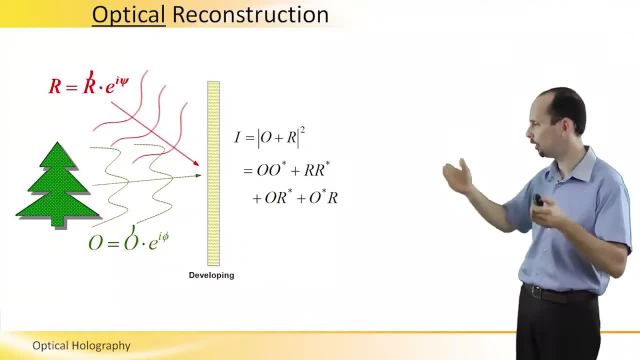 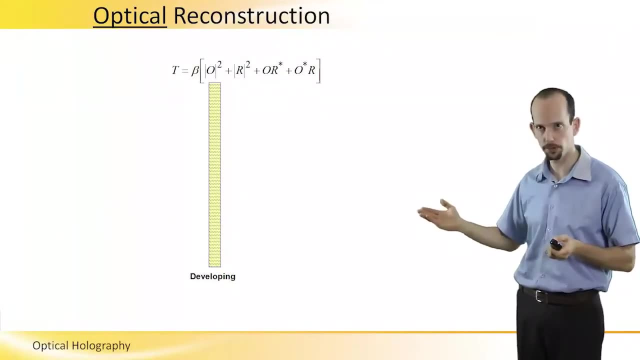 So we have recorded an hologram, a superposition between the object wave and the reference wave. But now we don't have the object anymore, We just have the photographic film. And I'm taking this film which captures these four elements. I'm developing it. so the transmission: 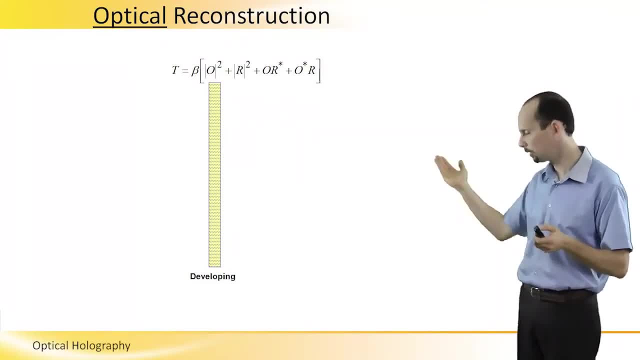 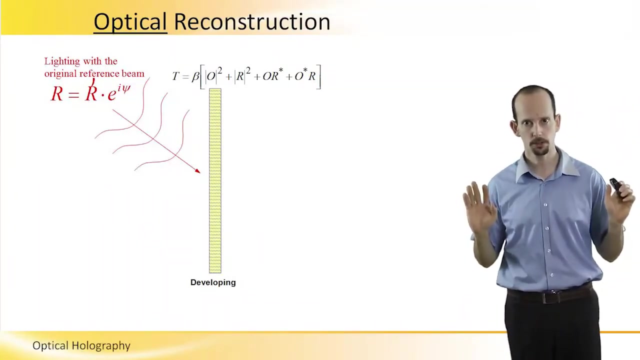 of this film tends to be these four elements multiplied by a certain constant which is dependent on the development process. And now I'm using the original Reference wave. I don't have the object anymore, but I do have the reference wave, which comes directly. 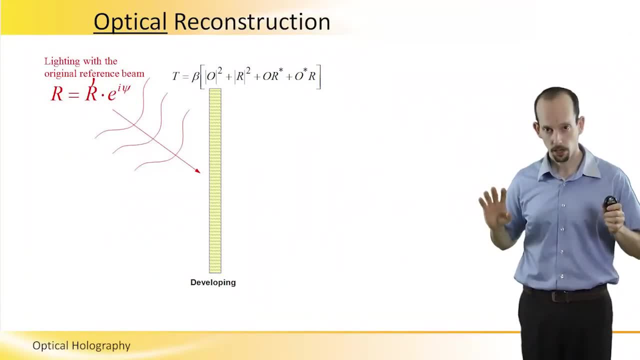 from the source. I'm illuminating the object- sorry, I'm illuminating the film- by this original reference beam. And this reference beam, when it passes through this thin mask, the hologram, actually means that the reference is multiplied by each of them. 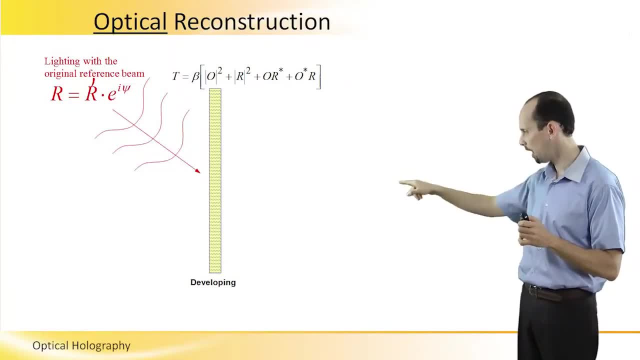 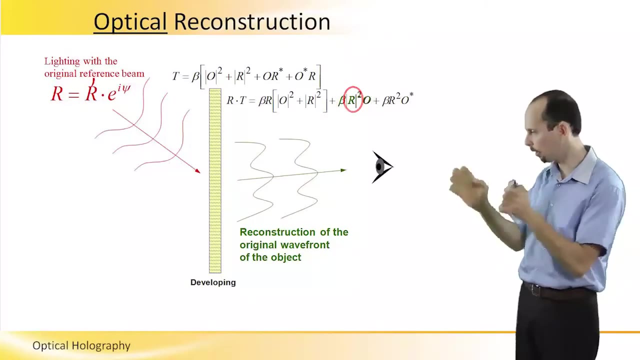 By each of these four elements And as soon as this r multiplied by the third element, r conjugate multiplied by r, tends to be an intensity. So I'm getting a constant multiplied by the original wavefront of the object that has an amplitude of the face. 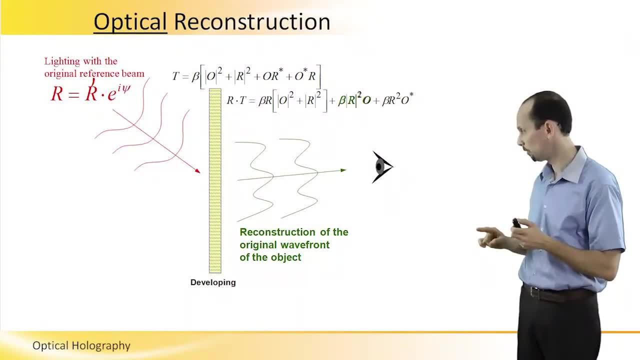 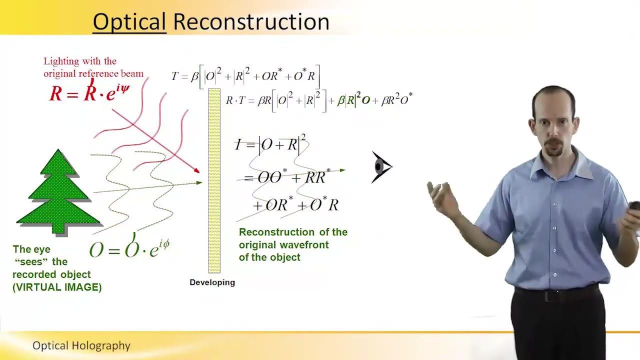 And the face. this is a complex number, So If My eye here Is in the right angle, I'm seeing only this element, And that actually means that I can see the original three-dimensional object inside the hologram, So the eyes actually see the recorded object. 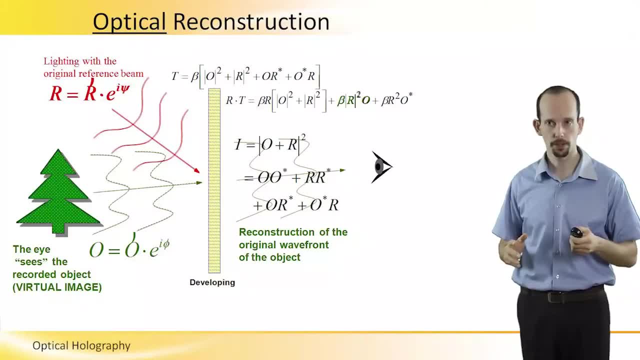 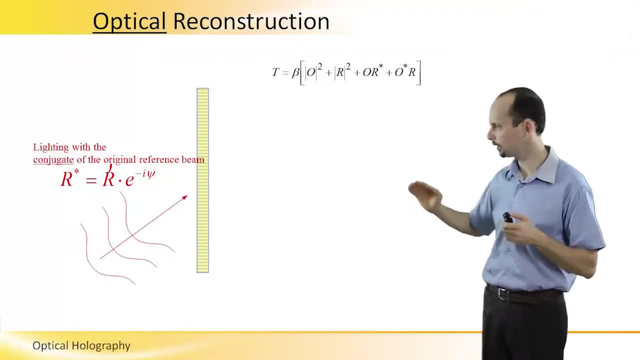 And because it is behind the hologram, it is called a virtual image. Now what happens if I choose to illuminate The hologram? that I have already recorded with the conjugate of the original reference beam. So I have here r conjugate. 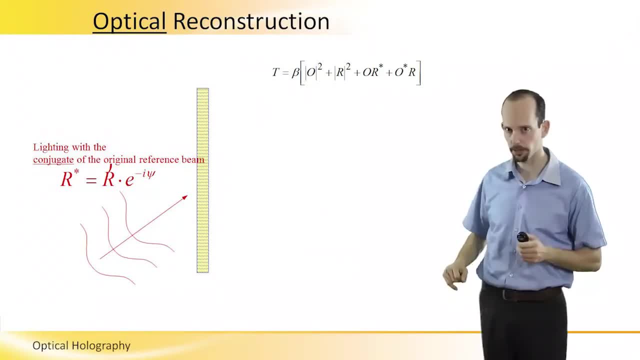 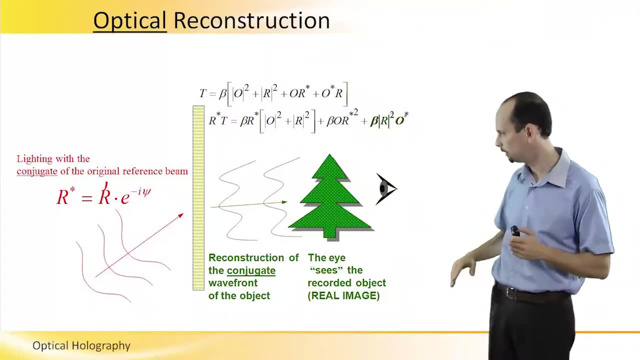 And because it's the conjugate, I have a minus here for the face. So as soon as this r conjugate hits the transmission hologram, I'm getting the four element, which is critical here. And If My Eye here 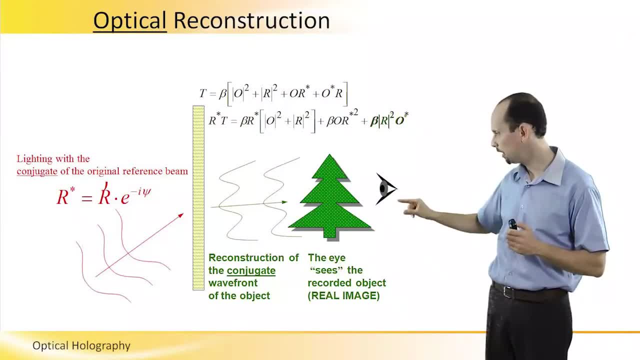 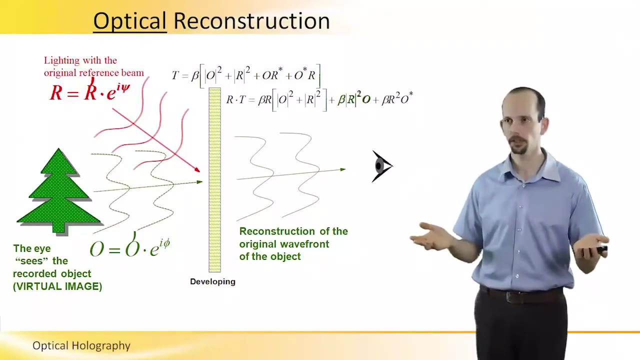 Is in the right angle, I will see the recorded object in front of the hologram plane. So this is a real image. So we have seen that in order to record an hologram, we need to record an interference pattern. We have seen that there is certain criterion, a certain feature of the source: long coherence. 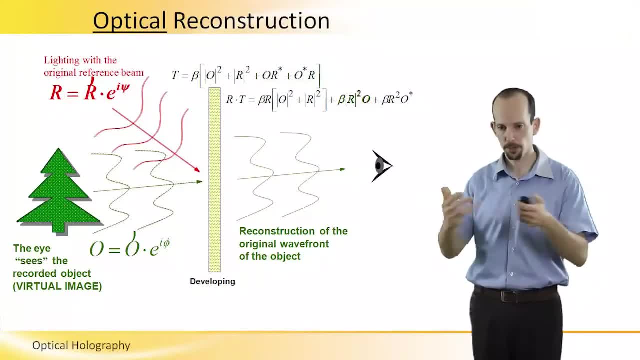 length for which interference pattern is feasible to be recorded. We have seen that a hologram, which is based on the interference pattern between the object wave- A wave that interacted with an object- and a reference wave coming directly from the source, is needed in order to create a hologram. 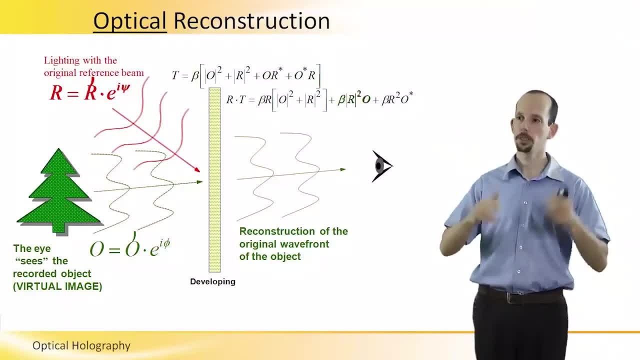 We've seen that the hologram can record the object, amplitude and the phase, which is the important thing, And we have seen how we can optically reconstruct the hologram. So Optical reconstruction mean meaning that I have the hologram already recorded optically. 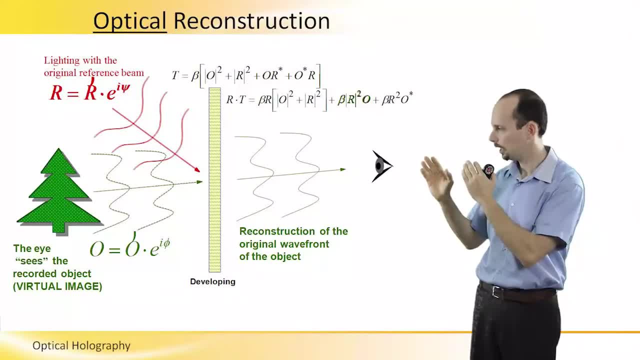 and I'm reconstructing it by illuminating the hologram optically by the original wavelength. This is why it is called optical holography. In the next section, we will see what digital holography means, which actually means that, instead of this photographic film, I'm going to use a digital camera and reconstruct the 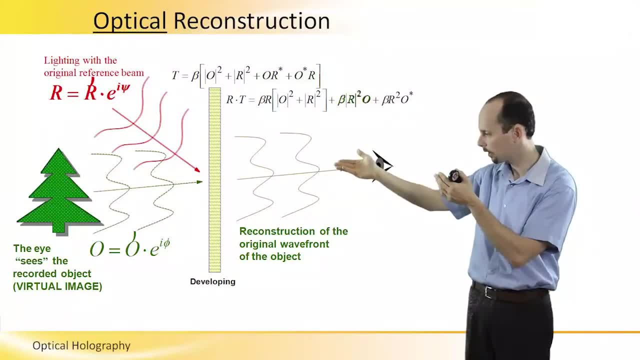 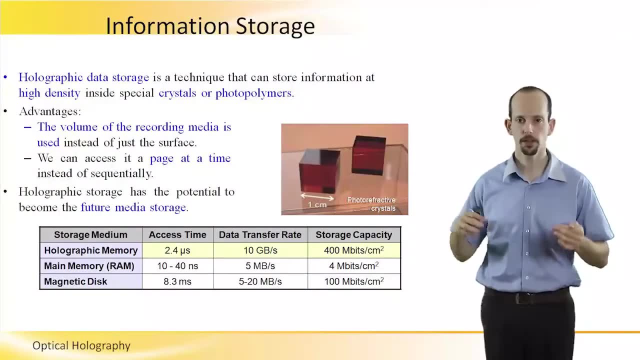 hologram in the computer Instead Using the original reference wave to illuminate the hologram. So before we are going to talk about digital holography, let's let me show you several interesting applications of optical holography. So the first one is information storage. 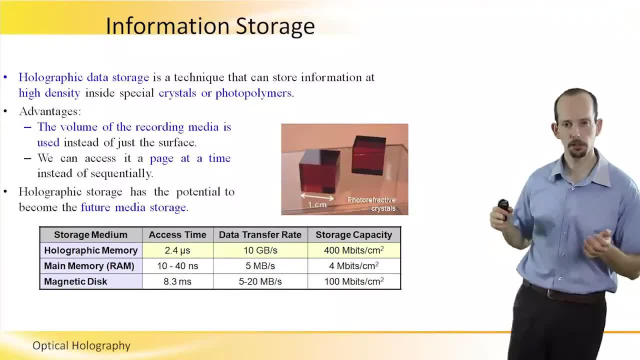 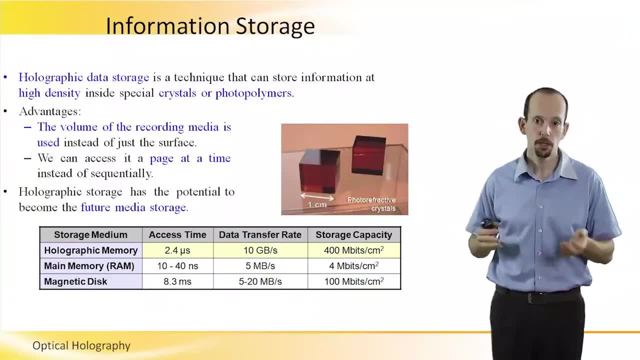 So holographic storage might be the future storage, information storage in the future, because we can use crystals Or We can photopolymers, such as photorefractive crystals, in order to create volume holograms, which means that we are creating holograms that are recorded in the depth of the medium. 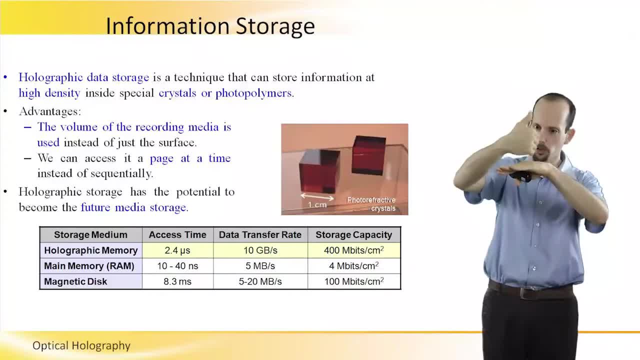 So it's not a thin hologram, It's a crystal for which I can record holograms in different angles, So I can actually store a huge amount of information. But the most important thing here is that the data transfer rate is much, much faster. 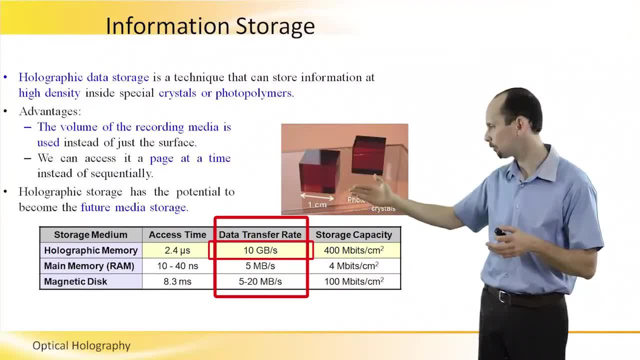 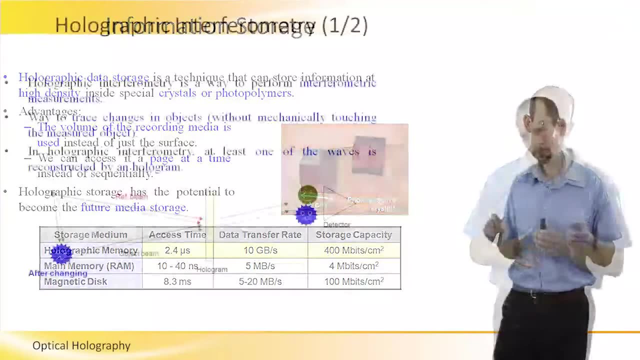 compared to RAM or magnetic disk, compared to the main memory of a computer and a magnetic disk. So I have here a very, very fast data transfer rate for the potential storage, information storage of the future. So the second application is holographic interferometry. holographic interferometry is a method to 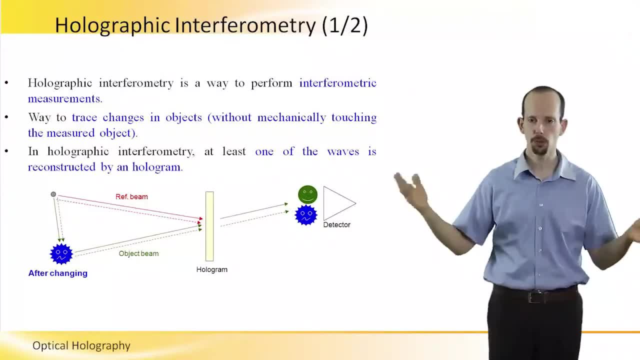 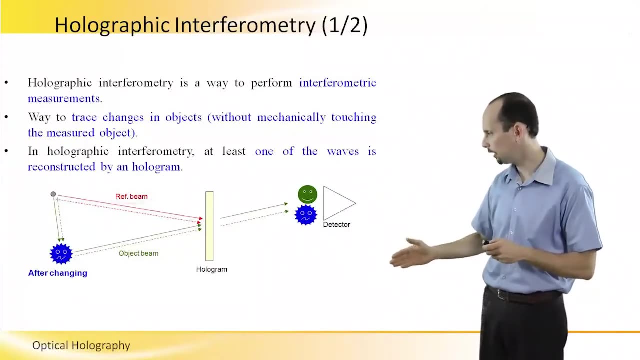 perform interferometric measurements and I'm able to trace the changes in objects without mechanically touching them. I just need to illuminate them by a light and interfere with the reference wave that come directly from the source, And then I'm recording the object before and after the change. 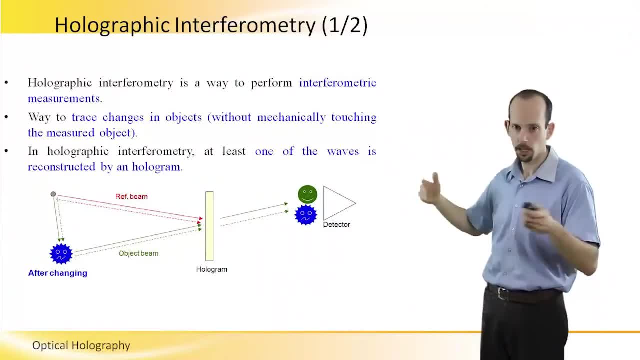 And then I can compare the holograms. or another way to do that is to record the object only once and to project the interference pattern or the hologram on the object in order to see the change in the object. So This is about holographic interferometry. 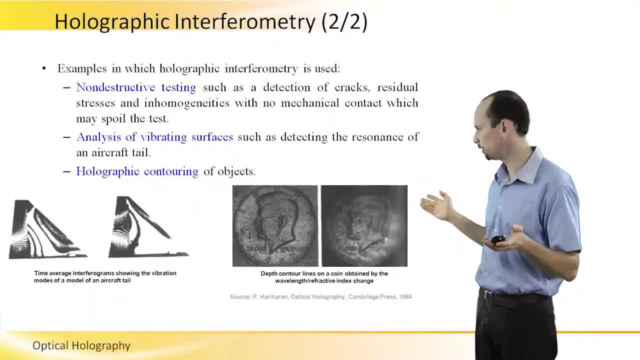 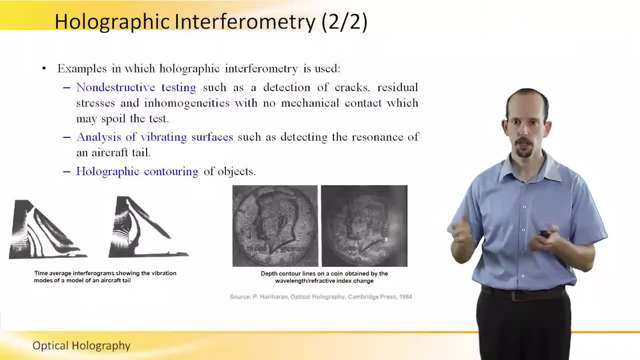 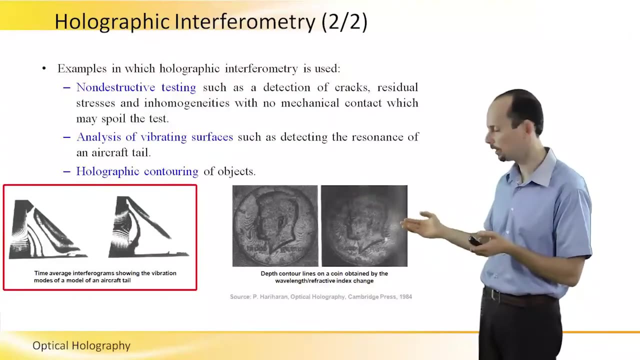 So, as an application for holographic interferometry, we can have non-destructive testing, such as detection of cracks and residual stresses, without mechanical contact which might spoil the measurement. As you can see, here we have a tail of an aircraft and we can actually record interferograms. 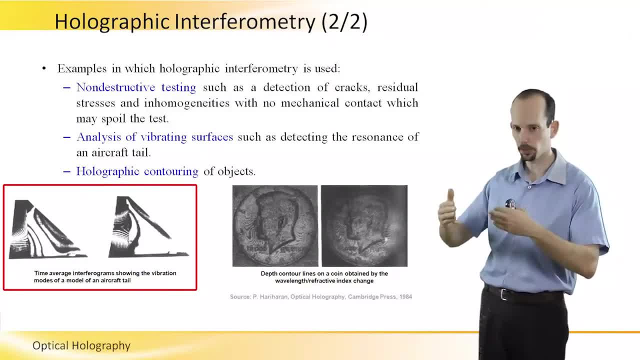 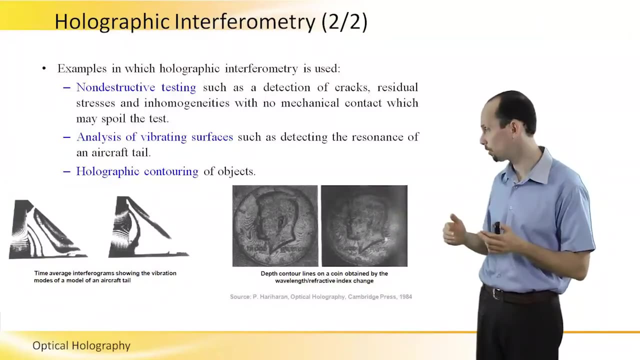 or holograms of this tail Before and after the change, and the tail is always vibrating, So we can see where there are cracks and residual stresses in this tail. We can use it for analysis of vibrating surfaces and we can use it for contouring of objects. 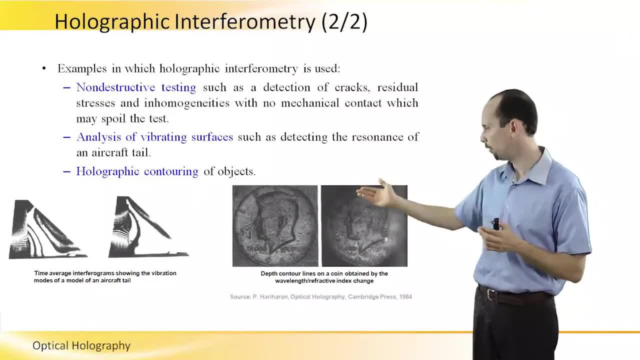 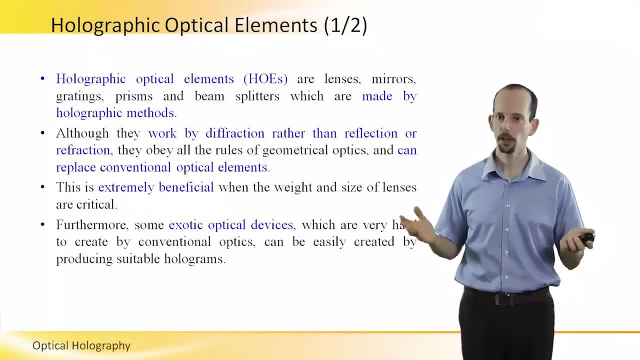 As an example, you can see here depth contours of this coin. The third application is holographic optical imaging. This is the first application of holographic optical imaging. The second application is holographic optical imaging. The third application is holographic optical observation. 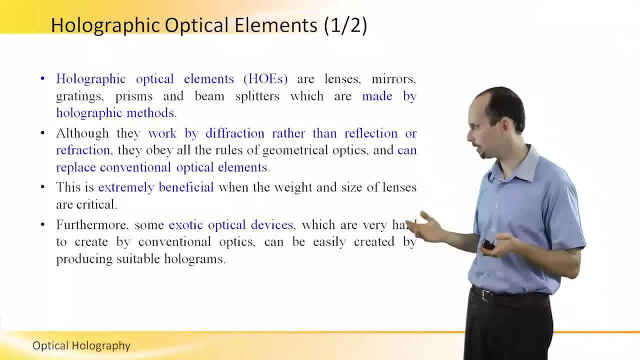 The third application is holographic optical imaging. But holographic optical images are an injectable harder mechanism. It is charged in a minimal capacity. each emission uses the스터 mut wallet, which is a final люди, And although responders do not require such means for surveillance, they are necessary. 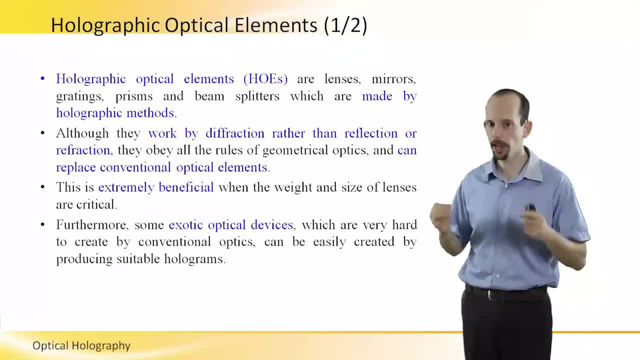 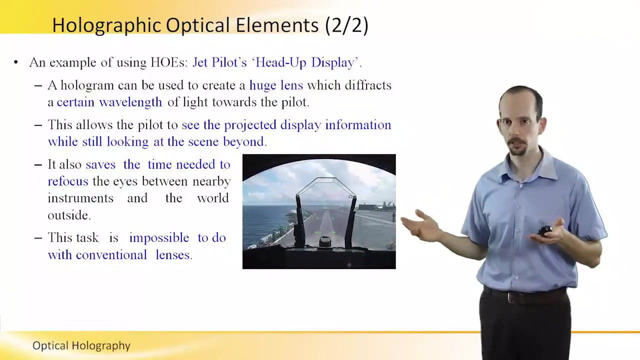 for the medical field That in no case requires more than everyone's praktic, careful experience- and Bob's. the size of the element is critical and in addition, it is possible to create exotic optical element which is very hard to create by regular refractive or reflective optic. As an example for holographic optical elements, you can see: 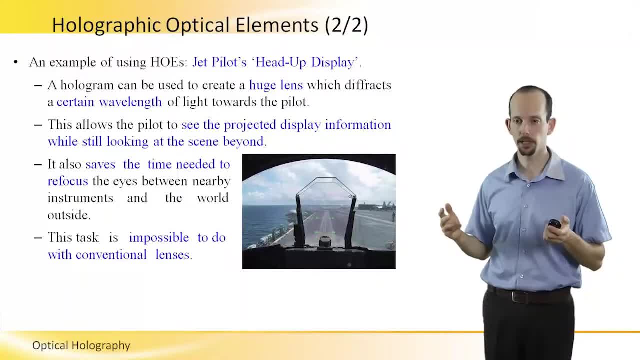 here this jet pilots head up display. so a hologram can actually create an effective huge lens which projects, for a certain wavelength, the display into infinity. so the pilot doesn't need to defocus his eye, he can see the display. you can see here the green digits. 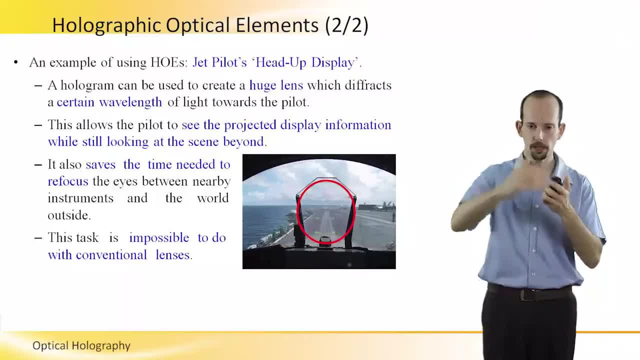 the display in infinity on the horizon, and it might be impossible to create this type of lens inside the is Hamlet, because this lens will be very, very large and heavy. Using optical elements- diffractive optical elements, holographic optical elements- this task becomes possible. The fourth application is: 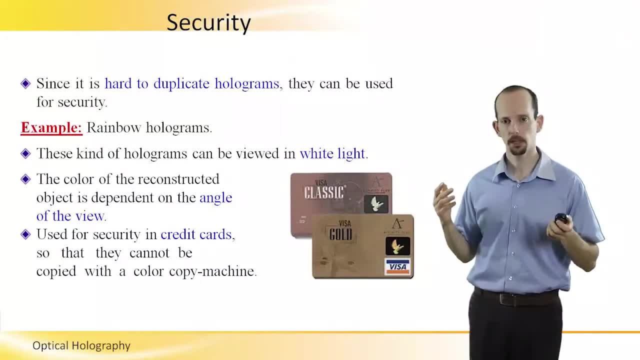 security. It is kind of hard to duplicate holograms. although it is not impossible, the person that has the negative of the hologram can actually reproduce them in large amount. as an example, we have the rainbow hologram, which you all know, which is well known from your credit cards, and this kind of hologram can be 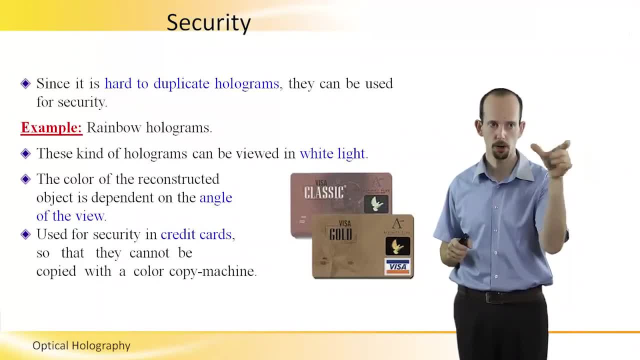 viewed in white light. if you take your credit card and move it horizontally, you will see the parallax effect and you can see that the hologram is actually moving. You will see a 3d image. but if you move it like that, you will get a. 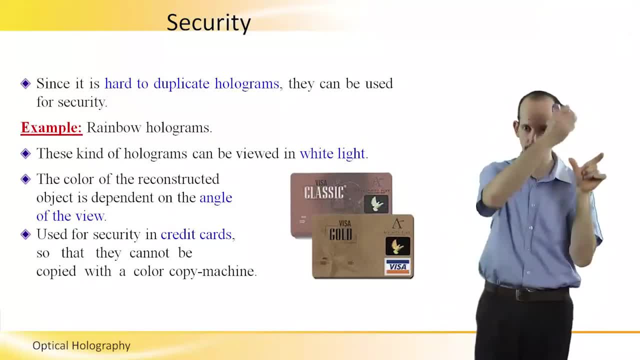 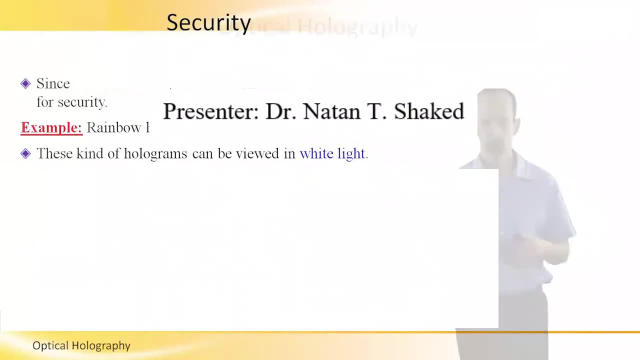 rainbow of colors, but you don't have parallax in the vertical axis and this kind of hologram is actually used for security in credit card, so that it is hard to be copied with regular color copy machine.